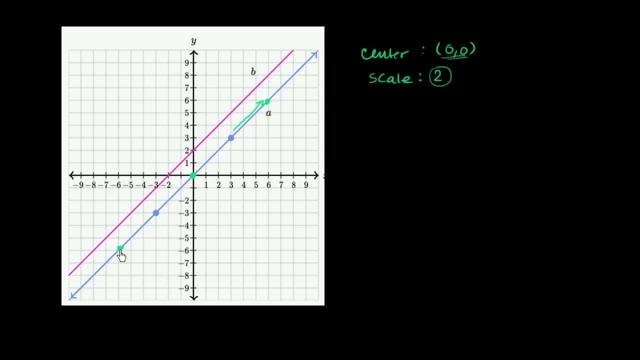 So it's going to be six less in the x direction and six less in the y direction. Once again, just pushed out. So notice, when we picked a center of dilation that sits on the line. it really doesn't matter what scale factor we pick. 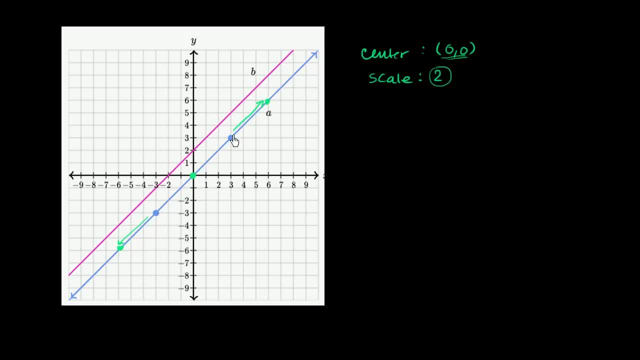 We'll just essentially be stretching and shrinking the points along the same line, And since this line just keeps going on and on and on forever in both directions, it's really just going to map onto itself. If this was a line segment, we would. 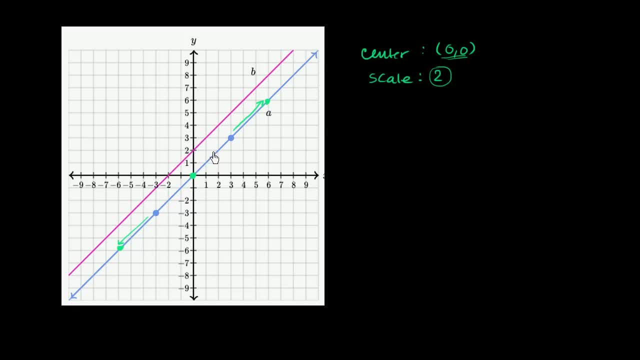 be mapping it to a different line segment that would have the same slope but its length would change. But a line has an infinite length, So as you stretch and squeeze it, it still has an infinite length And it's just mapping it onto itself. 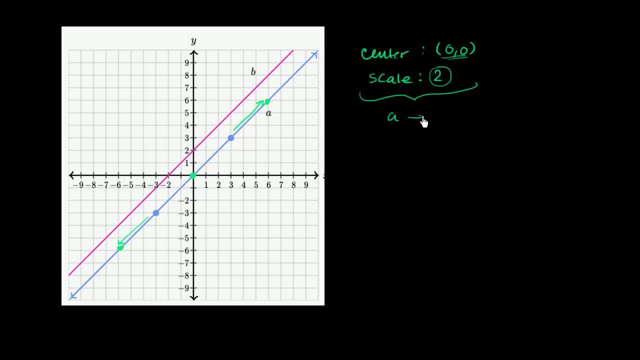 So this dilation right over here: a is going to map onto itself, It's just going to map onto a. So that's not going to suit our purposes. But what can suit our purpose is if we pick another point that's not on a and not on b. 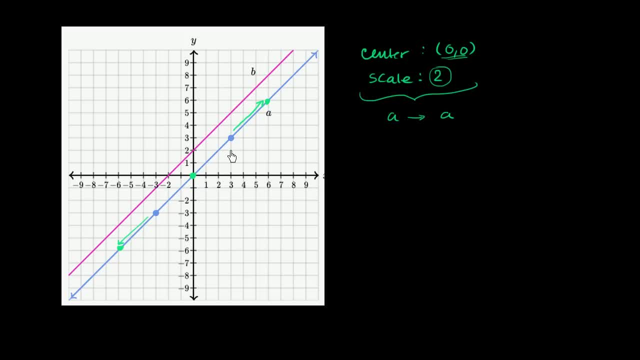 Let's say, we pick this point right over here And I like this point, And so let me pick that as my center. I'll tell you why I like it in a second. That is the point 3, comma 2.. The reason why I like that is we can. 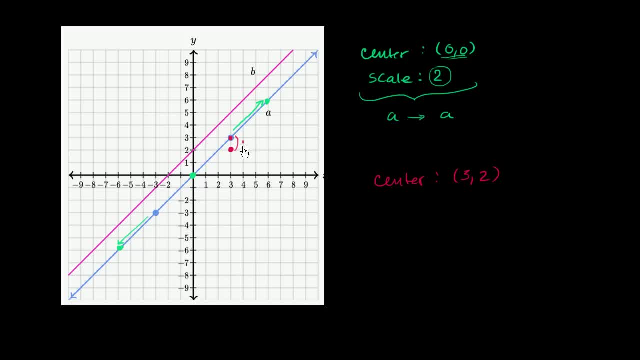 see that this point on point a right now is 1 away And if I want to map it to the corresponding point on point b, well that's going to be 3 away from our center of dilation, So I could have a scale factor of 3.. 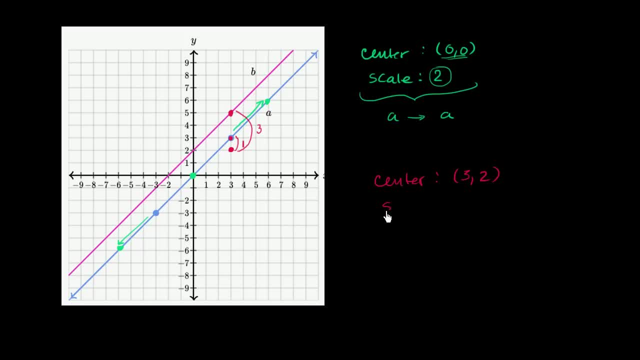 If I have a scale factor of 3, it's going to go 3 times as far away Scale factor of 3. And that'll work for other points as well. For example, this point right over here: It's 1 to the left of our center of dilation. 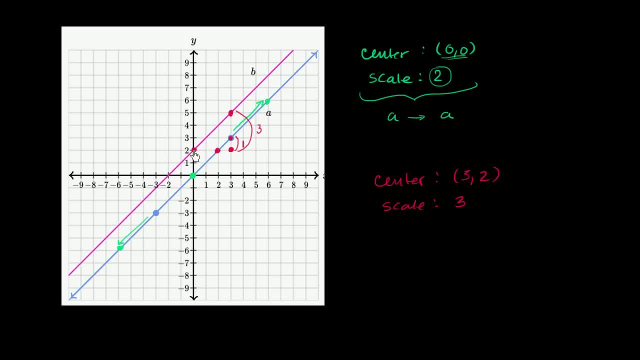 If we have a scale factor of 3, it's going to be 3 to the left, So it's going to map. If we think of it that way, you could think of it as going right over there. So I'm going to go with center at 3, 2.. 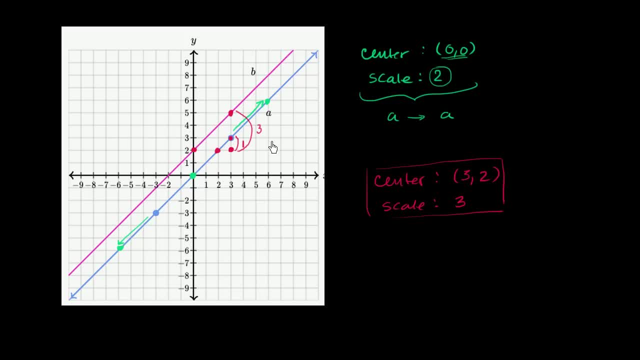 Scale factor of 3.. And you could have picked many, many other, In fact an infinite number of other centers, And then you would have had to calculate the appropriate scale factor for each of those. But I like this one because it fit nicely on the grid.